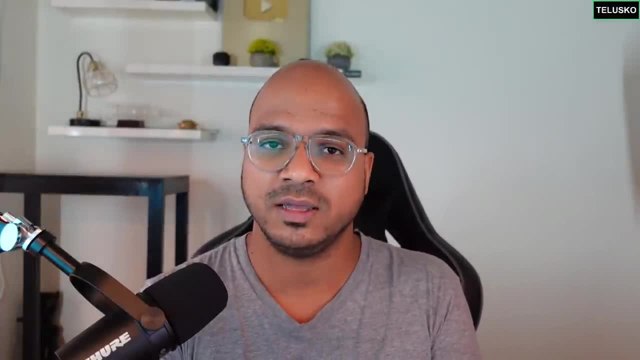 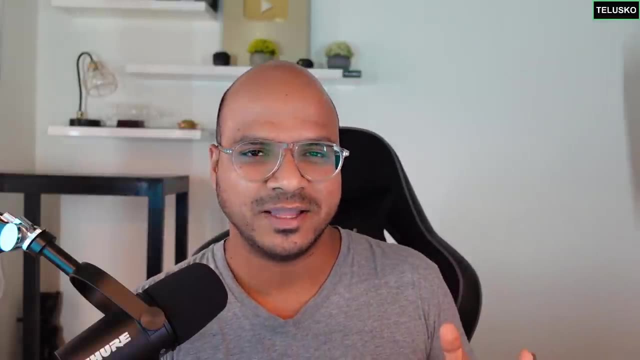 are living in a world of information right. The most important thing is information. now We have to secure data, but then we don't think about security. What we think about is just take the requirement and try to find a solution. So you will take the requirement and you will type the. 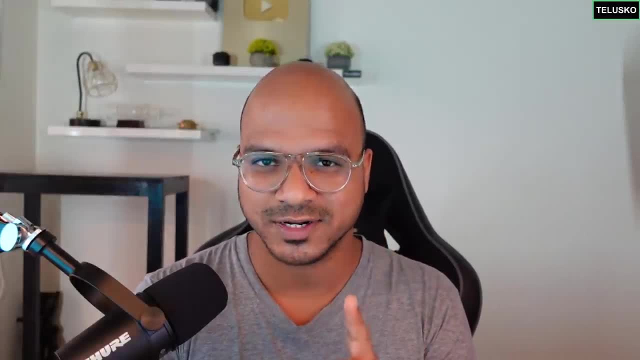 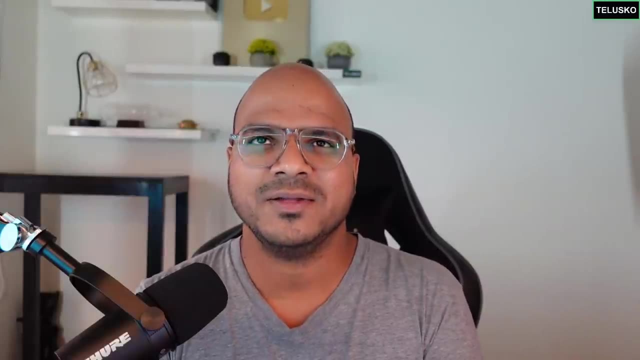 code. So the first parameter you have in your mind is: it should work, The thing which you do for your college work assignments and you know the final year project. But then, once you get into real world, when you get into a company, of course there are different. 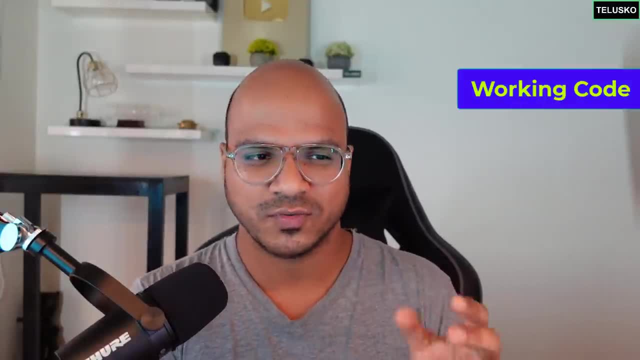 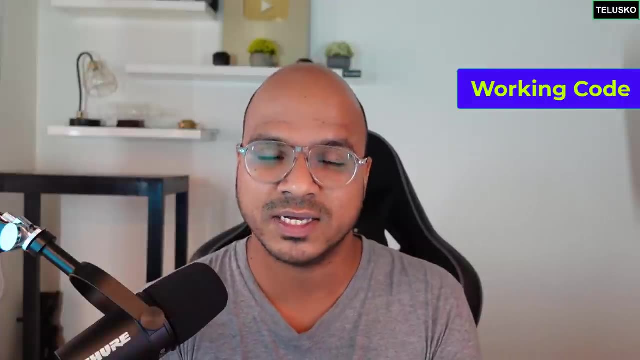 parameters you have to observe. The second parameter is, of course, your code should work. So when you write a code, of course that will be in your mind that this code should work, but also you want to make sure that your code, your software, is stable. Now, when I say stable, it simply means 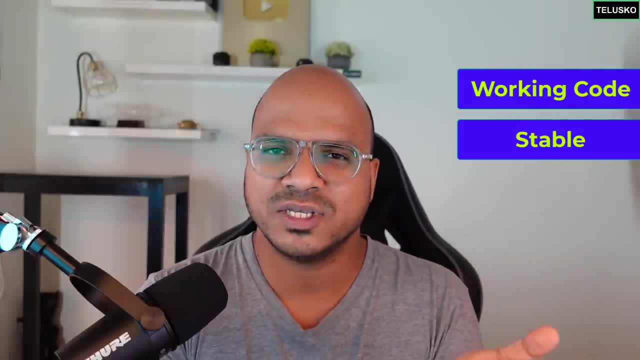 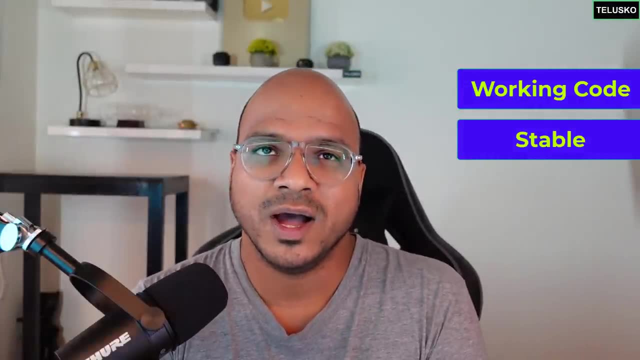 whenever a user is inputting a value, So your application is receiving some input from the user. if a user is giving wrong input or some input which is not Example- let's say, if you are asking file path but then the user is entering something else- Of course it will give you some exceptions. 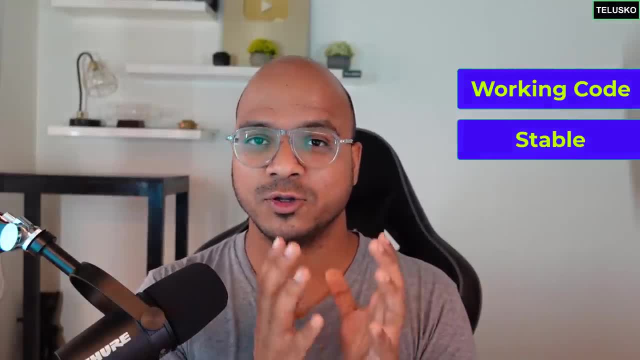 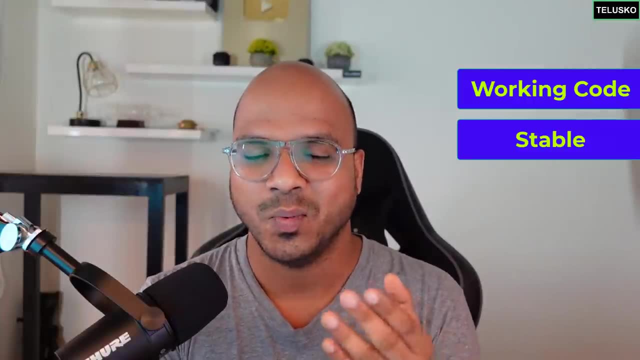 and most of the languages have this concept of handling the exception. So you should know that when you write a code, you have to handle the exception. You have to look for the all the parameters or all the boundary cases, What mistakes a user can make. So you have to handle. 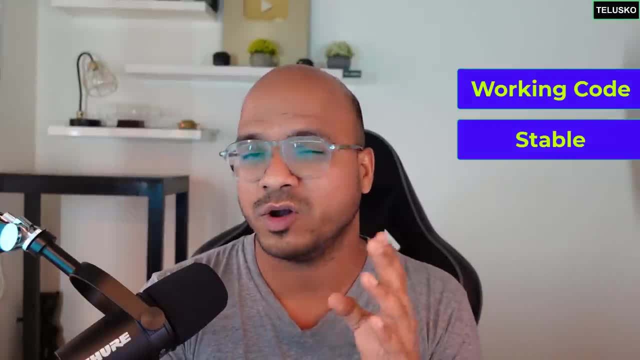 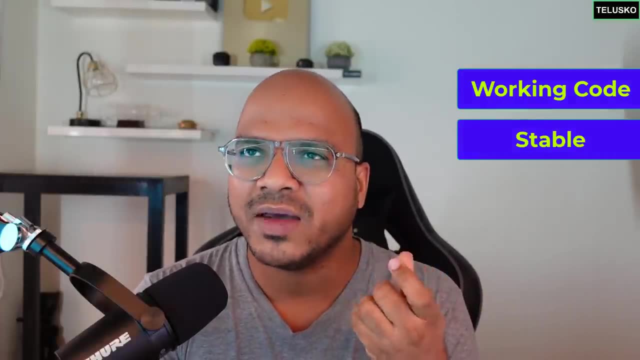 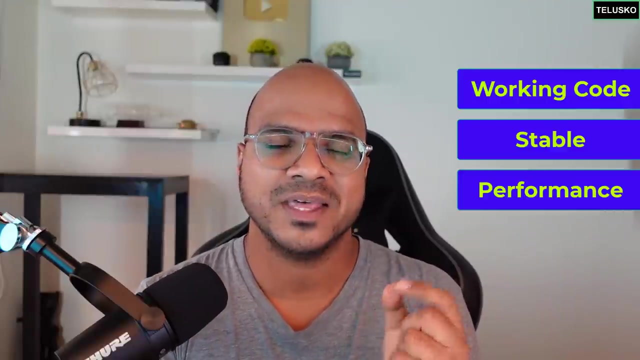 those exceptions. So two things: First, your code should work according to the requirements and second one, it should be stable. The next stage is depending upon your experience. of course, when you write a code, you will be having one more parameter in your mind, which is performance. Yeah, I want to build a application which will be fast. Example: 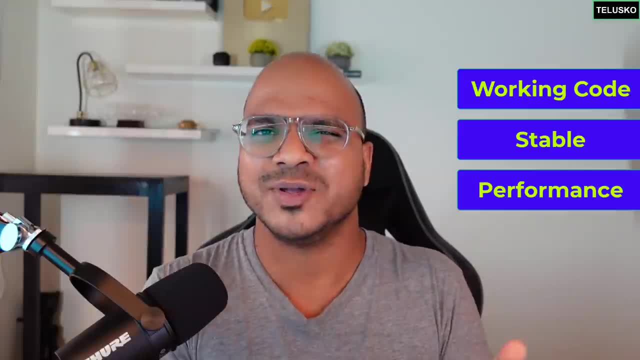 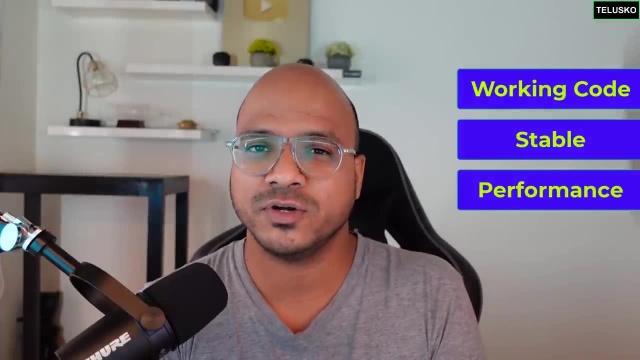 let's say, if you are going to a website and then when you click on a button, it something should happen, right? As a user, we don't have that much of patience, so it should be fast, Even if it takes some time for the server to respond. you need to do something to keep the user busy. Maybe show some. 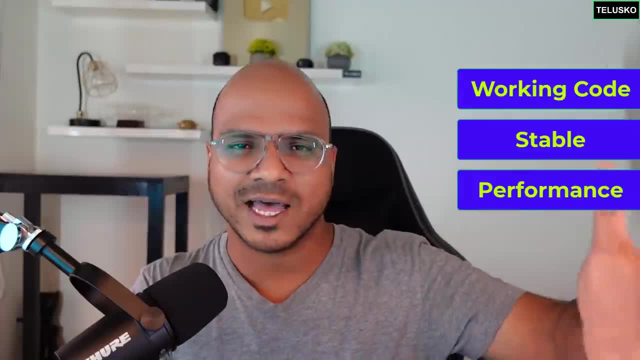 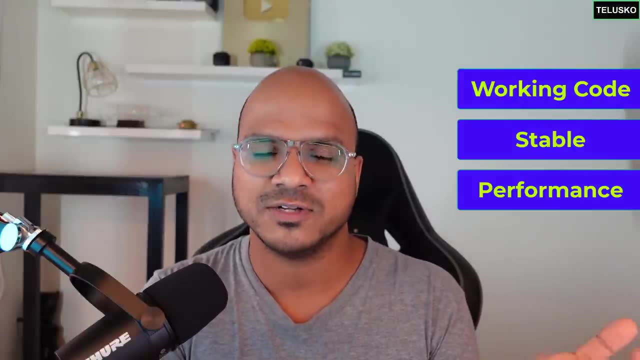 animations or, you know, tell the user something is happening behind the scene, but you have to do something. and even the response should be faster. User will not wait for more than a minute. That's my observation. So those are three things which are very important. right, The code should: 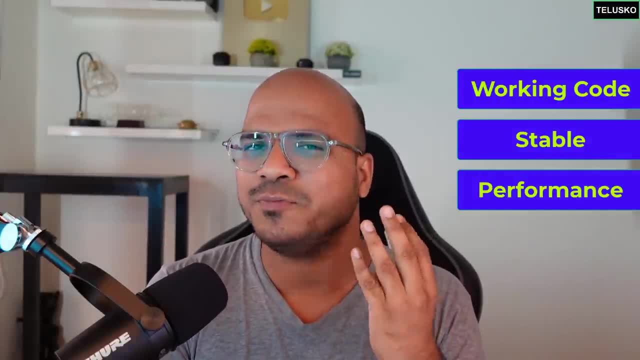 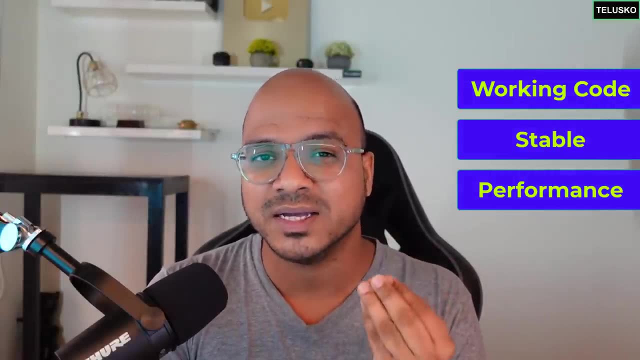 work, It should be stable, It should perform well. But the fourth parameter, which we always, always miss- In fact, I have seen most of the developers don't even focus on this thing- which is writing a secure code. You know why we miss this? because we all understand that whenever you build an 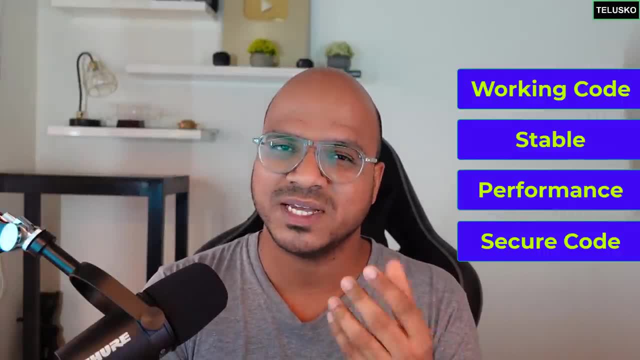 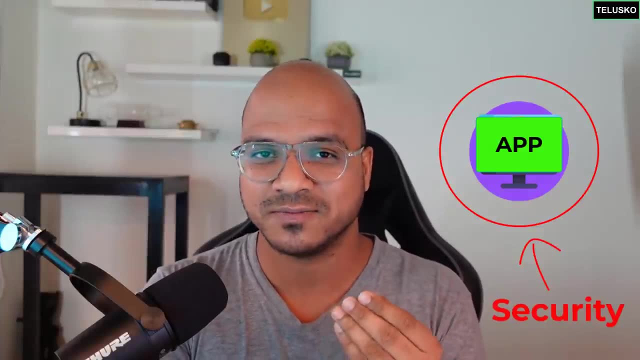 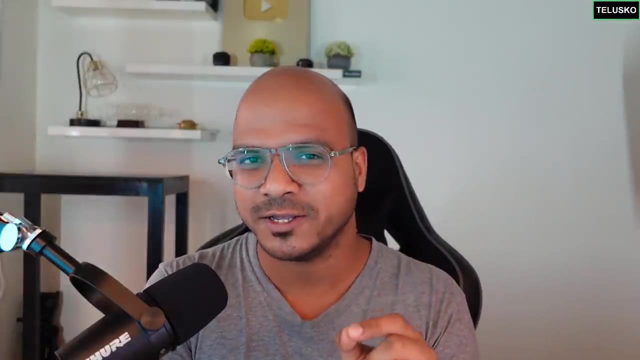 application. it should be secure. But the only problem which I see is we imagine as a developer, as a programmer, we imagine that the security is not concerned. There is a separate team sitting there to provide the security. See, there are two things here. One is application security and second is secure coding. When you talk about application, 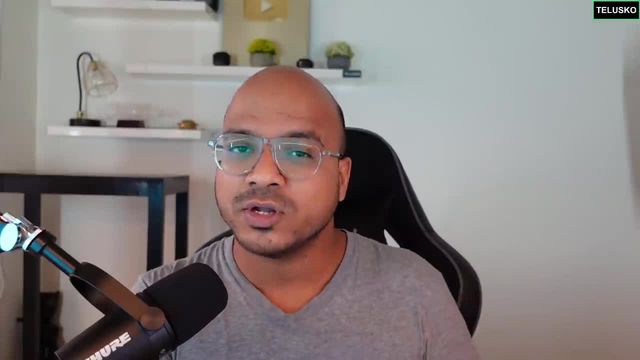 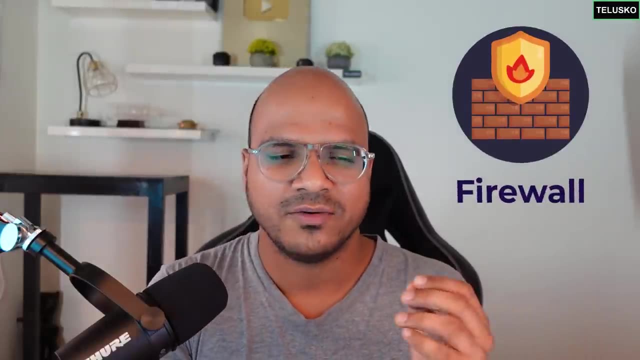 security. you are providing external security to the application, Something like: let's say, you have a web application and you want to provide security. Maybe you will say, hey, there's a firewall, We are having authentication libraries, so maybe you can use. you can verify username, password and all. 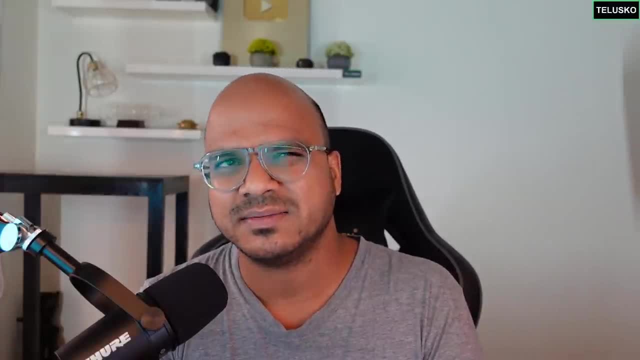 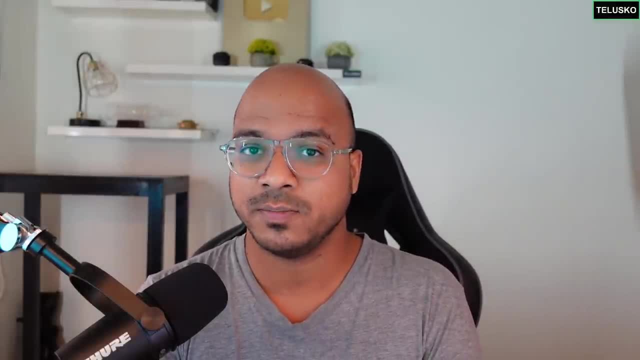 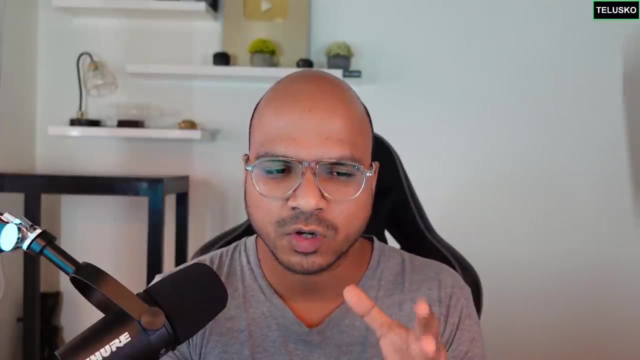 the application and what are their permissions, which are very important. But what we don't see is in your code itself, of course, whenever you write a code, there is always bugs in your application. I always say this and it is a fact. right when you say debugging is removing, 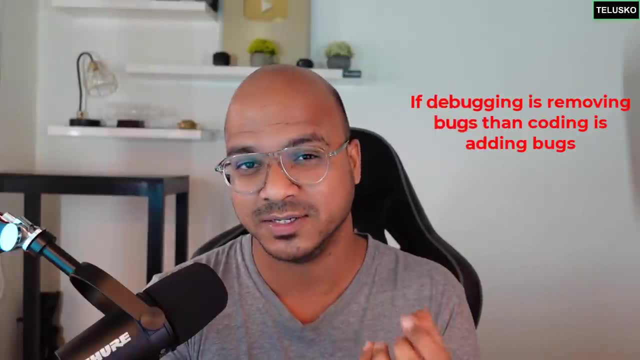 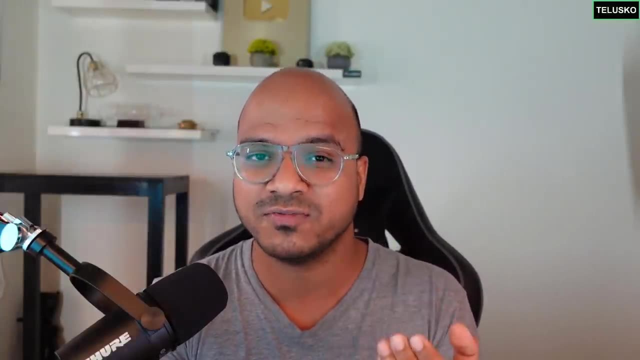 bugs, then coding is adding bugs. Of course in your application you will be having bugs. We have to reduce the number of bugs. See, some bugs will affect the stability of the application, some bugs will affect the performance of the application and some bugs will affect the 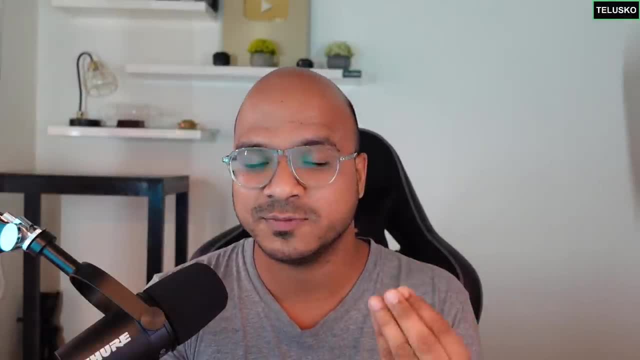 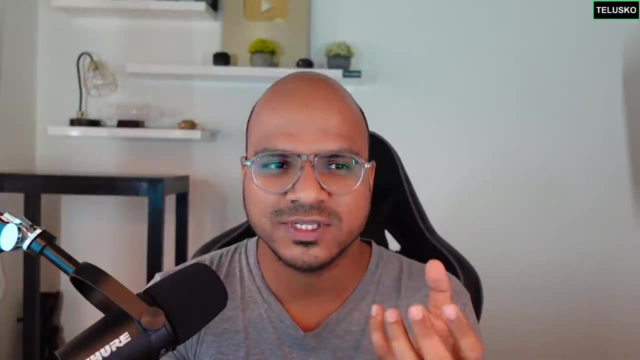 security of the application. so if you have a bug, your system is basically vulnerable. so you have to make sure that you don't have any flaws in your system. one of the way you can reduce that is by using smart packages or example. let's say, in java itself there are so many classes for the same. 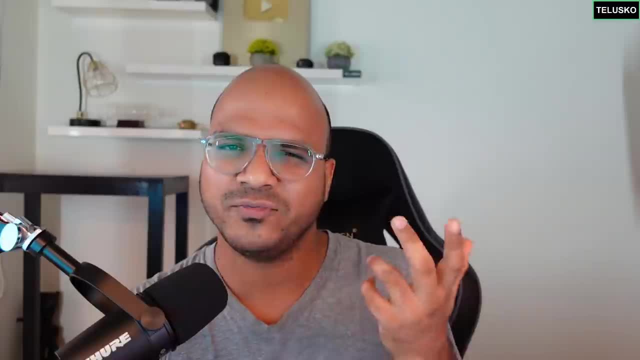 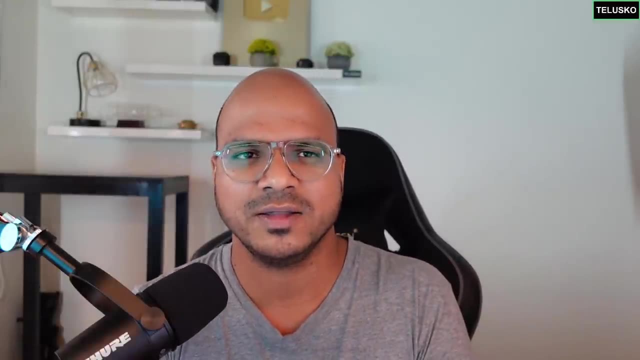 thing. so when you compare two classes and then you you say: hey, why we have two different classes for the same thing, then your teacher will say: hey, one is faster than the other one. of course that makes sense, right in the same way when you talk about security, when you write a line. so let's say: 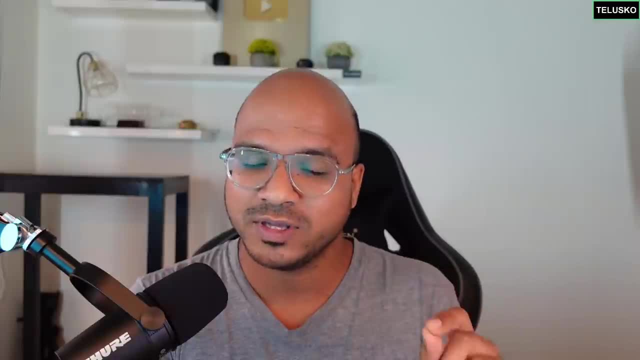 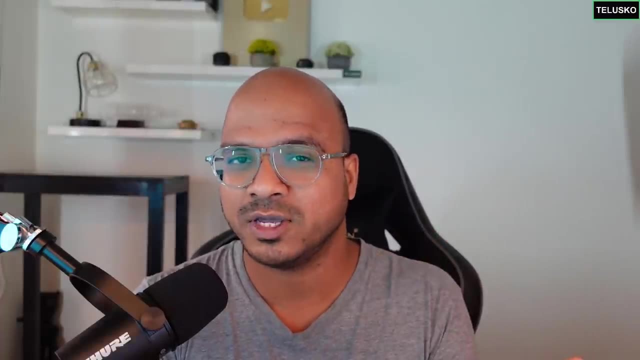 you are on line number five. this is a point. are you thinking about security? that's important. so even a simple keyword, you have to think about it. is this code secure? when you try to print something on the console, you have to think about it. is this code secure? so here we are not talking. 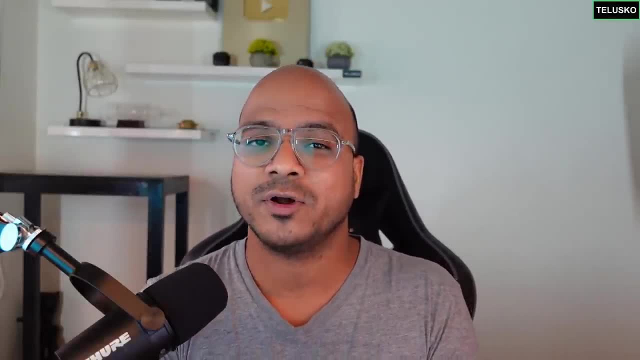 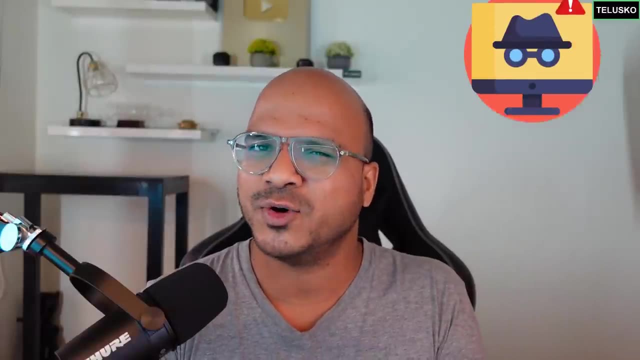 the external level of security. we are talking about the code which is secure. so when you write any line of code, make sure that you're not writing any code which will be vulnerable. so there are a lot of attacks which are going on right and then sometimes we don't. 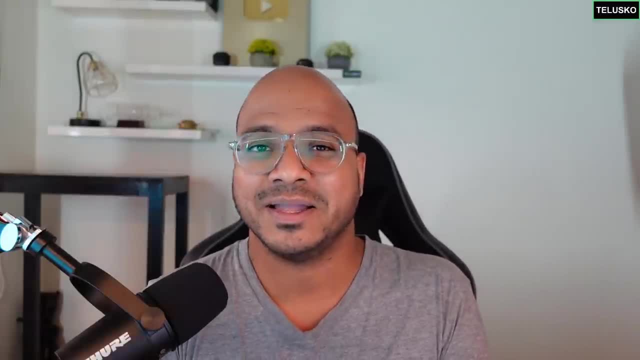 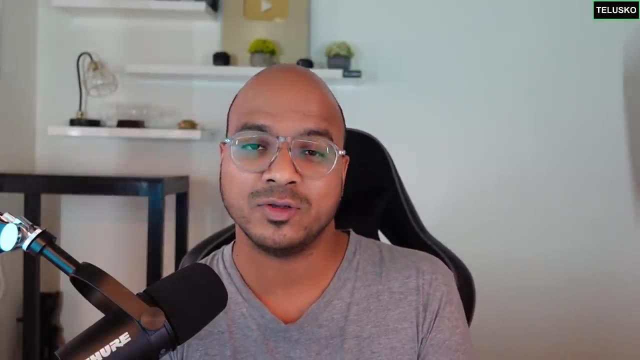 we are not concerned about the attacks. example: there's a data leak somewhere. every day you will hear some news from this server. this many data got stolen and now they're available on dark web. most of the news does concern us, but example: let's say, if someone says there's a attack on 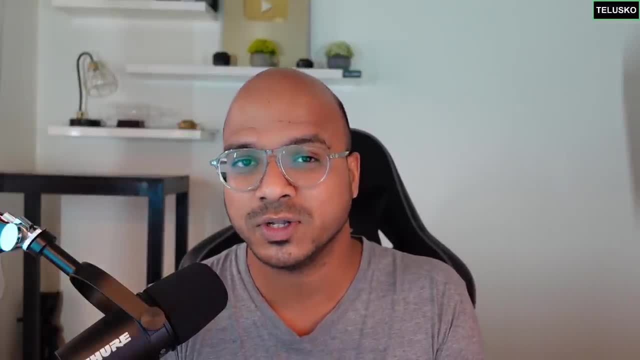 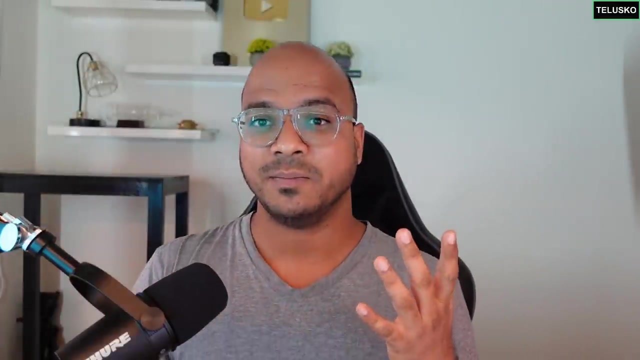 visa server and millions of credit card information got stolen, you will be a bit concerned, because money is important. example: bank account got hacked- you will be concerned. but if someone says, hey, millions of personal data got hacked, you will not be that much concerned. someone says, hey, there's a. 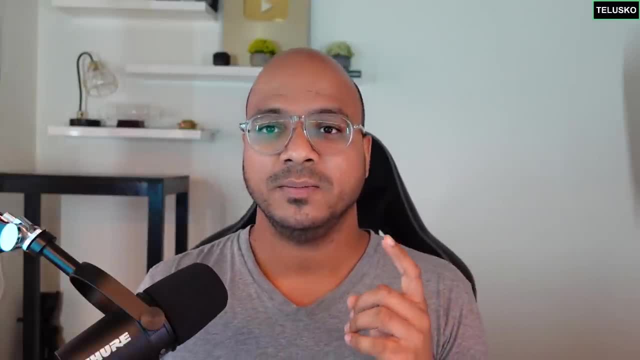 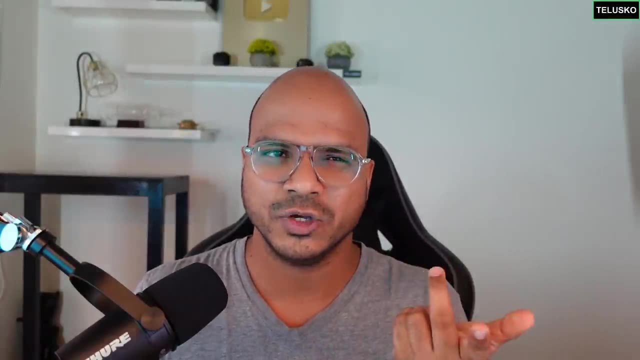 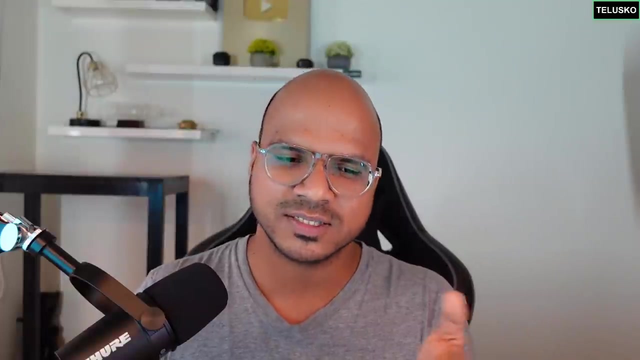 medical data which got leaked. you will not be concerned, right. but we have to be concerned about those things because see if you, if credit card got stolen, you can block the old one. you can get a new one. you will get a new number. if your bank account is getting hacked, you can block the account. there are some restrictions. 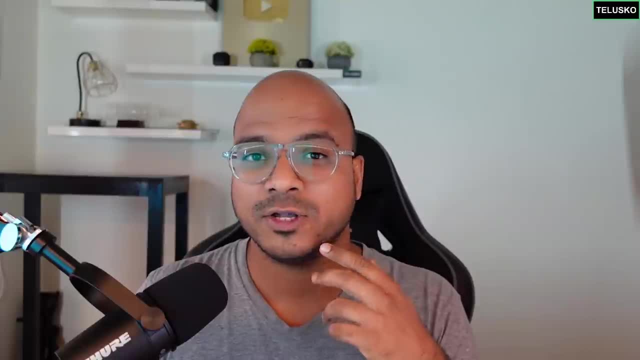 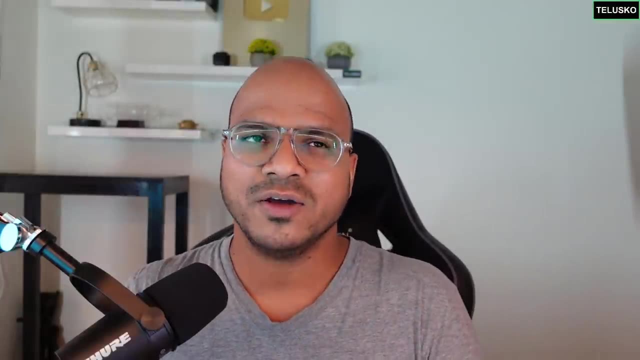 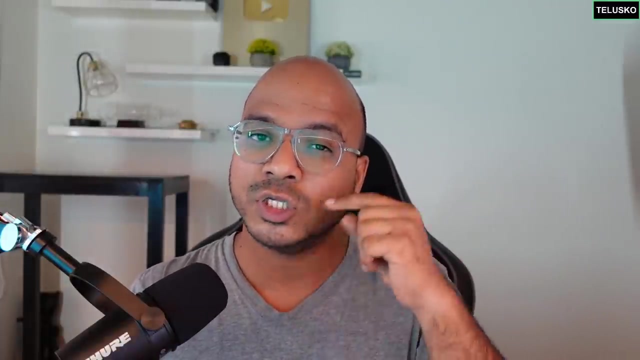 right, you can have a different bank account. what about medical records? what about your personal information? nowadays, data is very important, so a lot of companies are paying to buy that data on dark web. so you have to secure user data as well. so, even if you are not concerned about your data, you have to concern about the user's data which you hold. 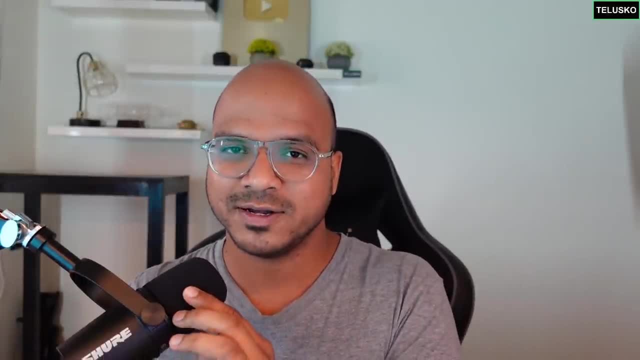 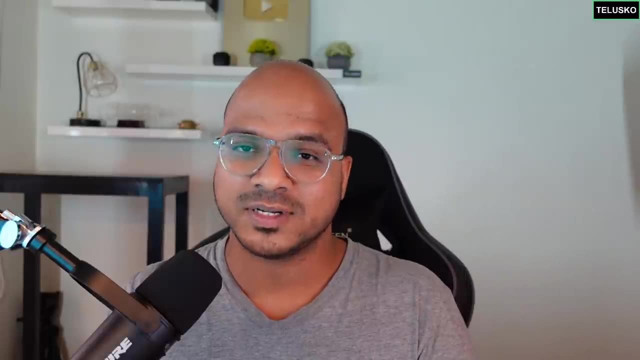 that's your responsibility and, by mistake, if you come under jdp, you will be fine. there will be a huge penalty and you might go to jail for not saving the user data properly. so you have to make sure that you write the code which is secure. now, what are the examples? 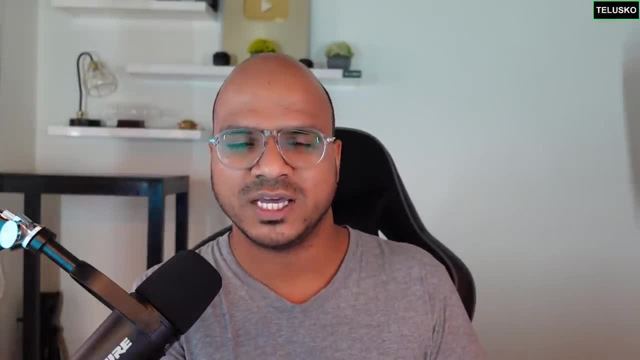 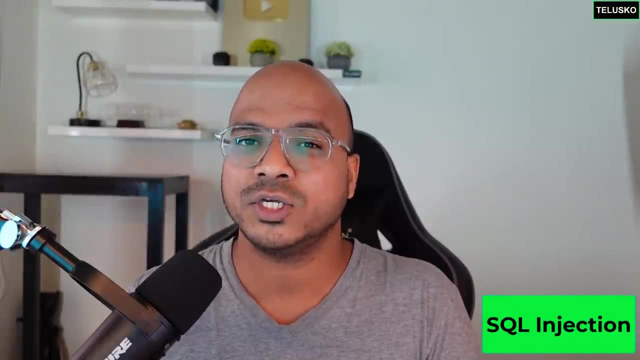 here just to make you understand. of course i can't teach you secure coding in one session. but example: let's say, if you talk about sql injection, it's one of the example of how can you write a secure code. you can stop sql injection. example: in java we use jdbc, right in jdbc we have 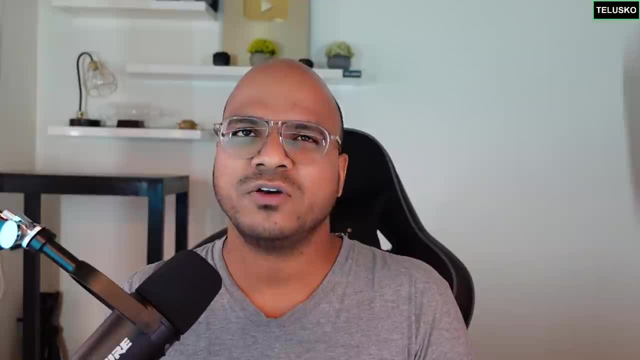 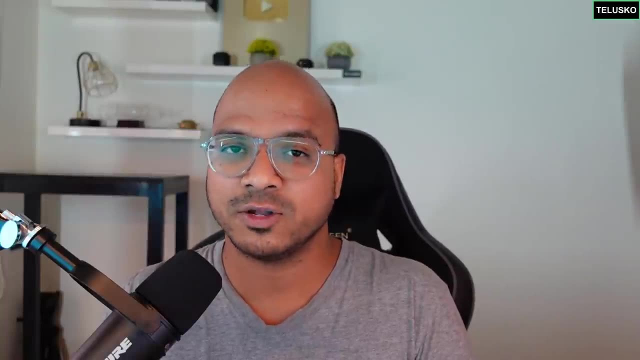 a concept of statement to write the code which is secure code, which is secure code, which is secure code, query instead of using statement. what if you can use prepared statement? if the values are coming later, it will make sure that it will stop sql injection. you know these things deserve a separate. 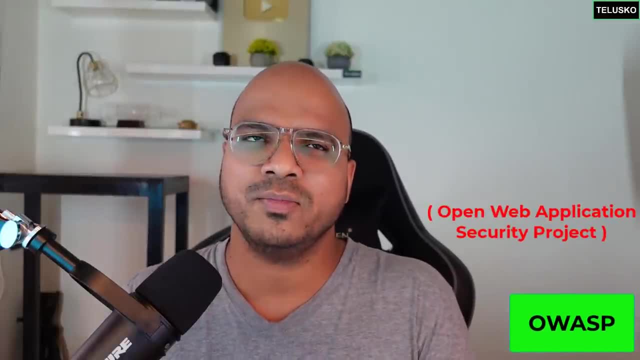 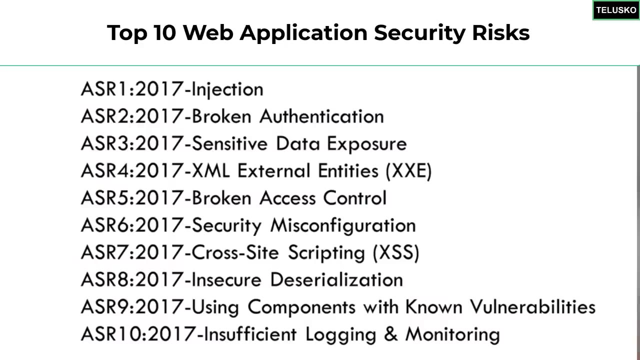 video. uh, so there is. o was pronouncing it right. they mostly focus on the web application security. you will find the link in description. so there are top 10 issues which they have listed. of course, there are so many issues available, but this is top 10.. of course, as i mentioned, 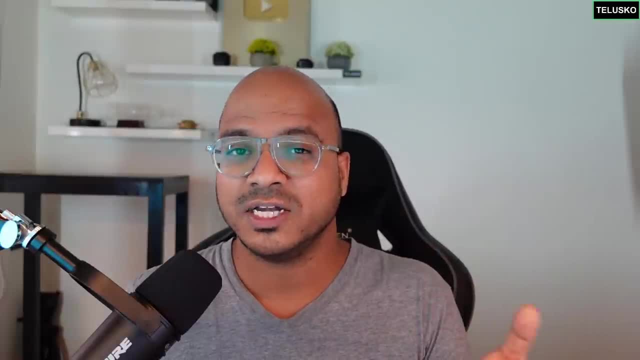 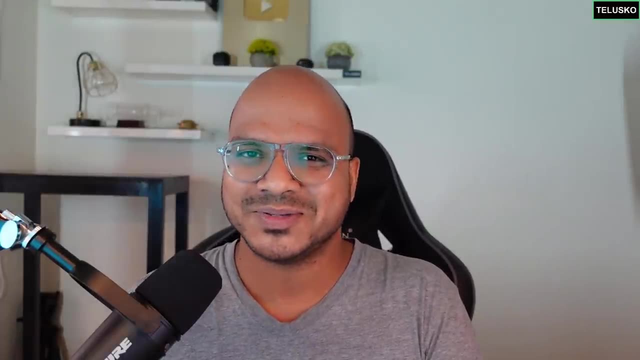 this deserve a separate video. so that's one of the thing: sql injection. the next one is: what if, if i'm whenever you send a data from server to client, is it secure? Is it encrypted? We don't think about those things, right, But make sure that whenever you do a transfer of data from server to client. 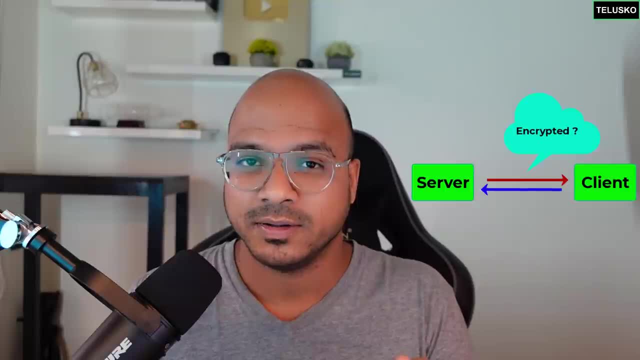 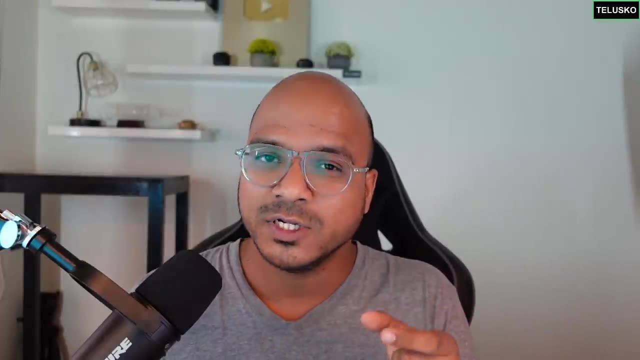 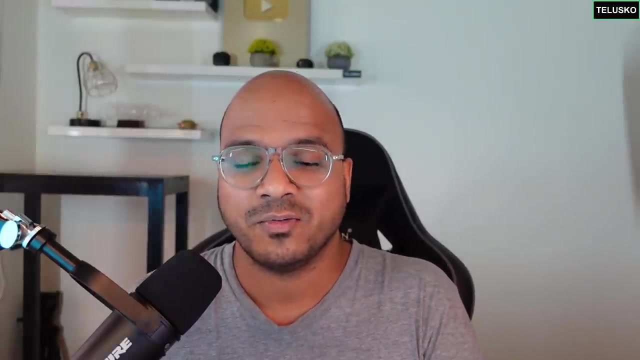 or client to server. is that data encrypted? Next one: let's say, if you receive a JSON from the client and then, of course, on the server side, are you able to process that JSON properly? What if there's a command? there's a Linux command in that JSON file. What if it is getting executed? 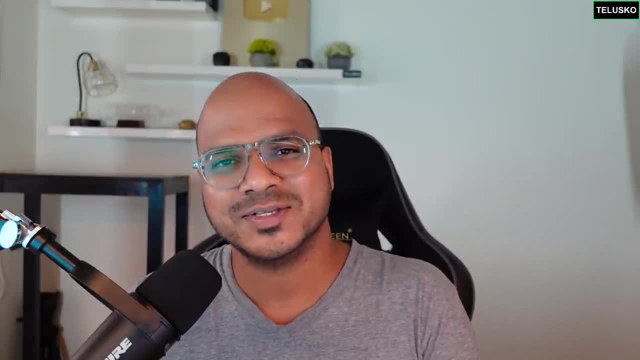 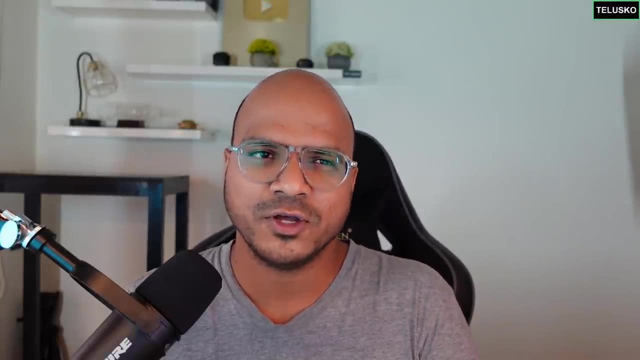 on the server Right. So you have to consider all those things. There's also cross site scripting, So you have to take care of that as well. Let me know in the comment section if you need a separate video on all these topics. I will try to make, But what is important is next time you write. 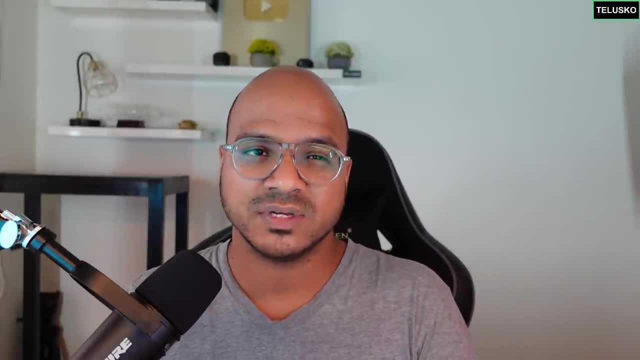 a code doesn't matter. Is it for your assignments? Is it only for learning a language? Make sure that you choose packages, you choose number of lines or the classes, based on thinking about security. One other thing I forgot to mention. you know most of the 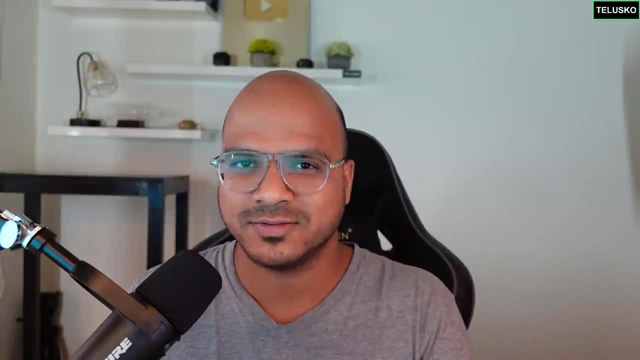 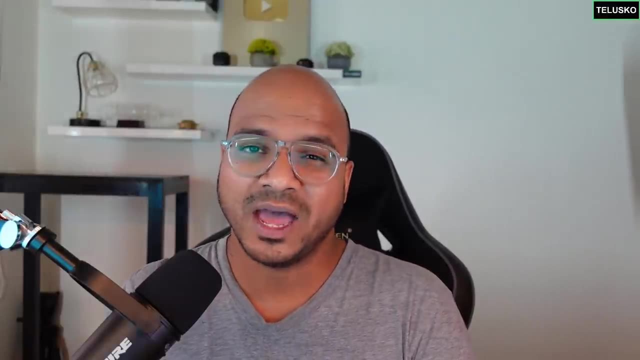 application which we build, we use some external libraries, right, Of course, if you say your project has 1000 lines of code, you can think about your project maybe having 10,000 lines of code, most of it coming from the libraries. So, whatever library you are using, are they secure? 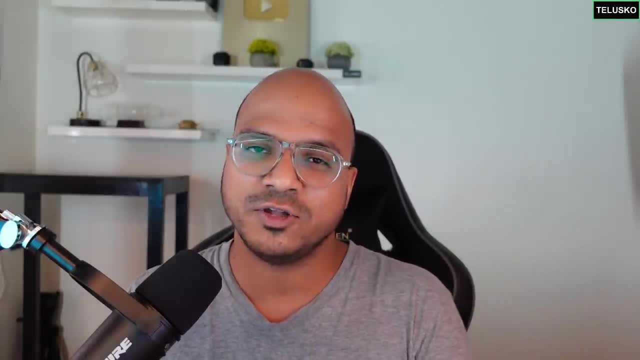 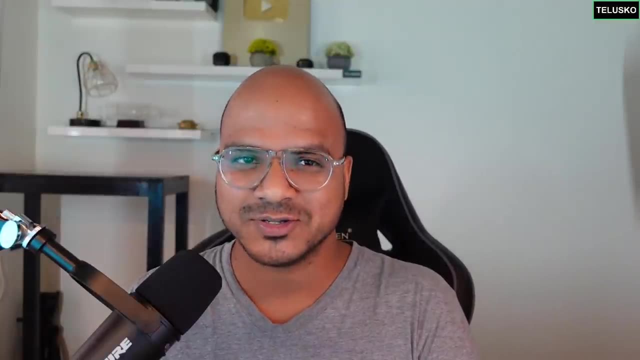 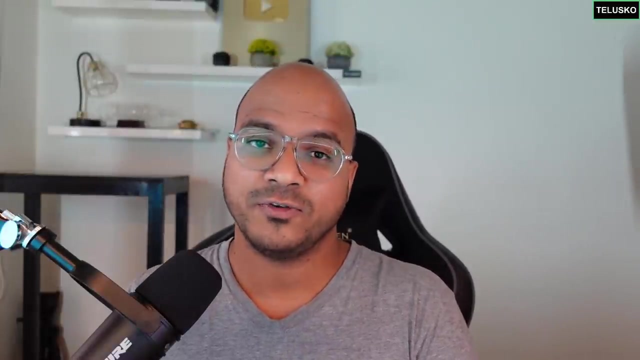 Even if your application, your code, is secure, the application which you're using might not be secure, So you have to think about those things as well. We have this habit of using beta libraries. don't do that. So yeah, if you want to learn, if you want to experiment, it's completely fine. But if you're